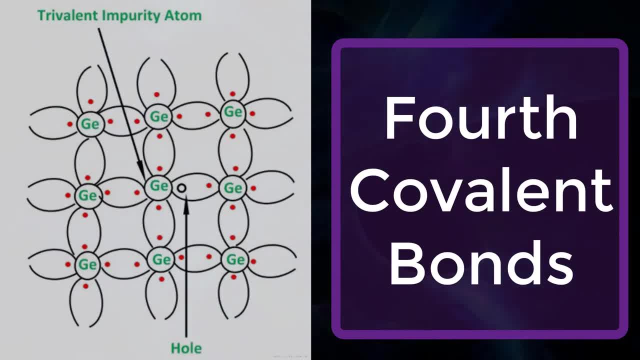 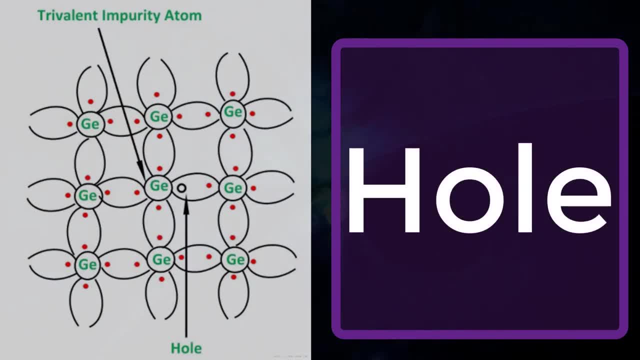 gallium atoms have no valence bonds, Hence the fourth covalent bond is incomplete, having one electron. short, This missing electron is known as a hole. Thus each gallium atom provides one hole in the germanium crystal As an extremely small amount of gallium impurity. 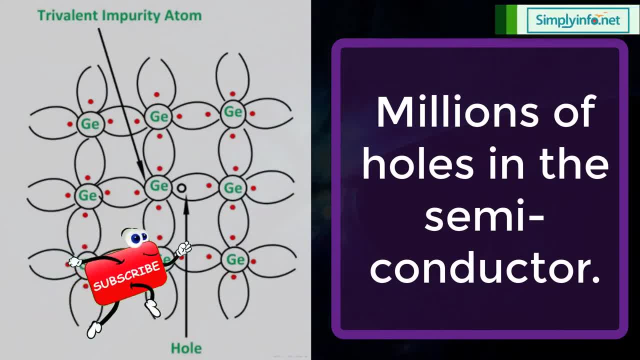 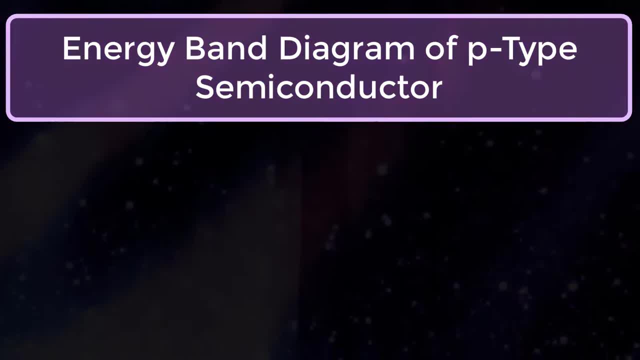 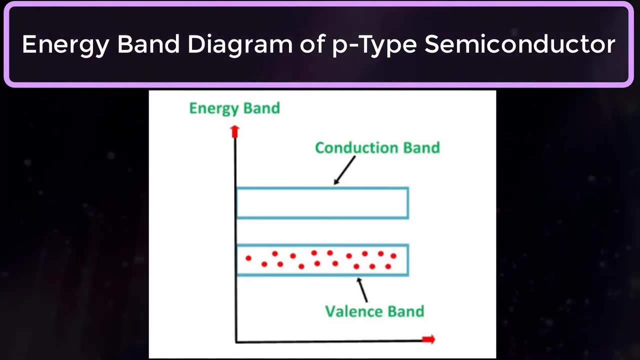 has a large number of atoms. therefore it provides millions of holes in the semiconductor. Energy band diagram of P-Type Semiconductor. The energy band diagram of a P-Type Semiconductor is A large number of holes or vacant space in the covalent bond is created in the crystal. 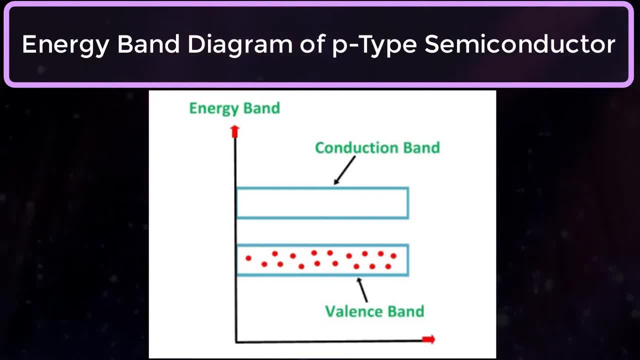 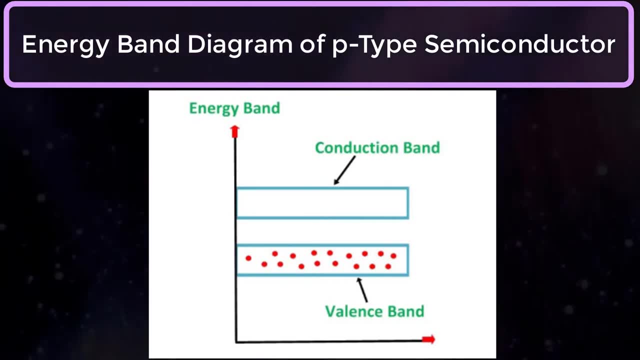 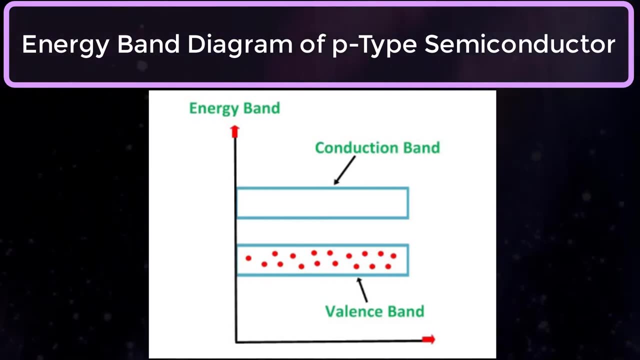 with the addition of the trivalent impurity, A small or minute quality of free electron is also added in the conduction band. They are produced when thermal energy at room temperature is imparted to the germanium crystal, forming electron-hole pairs, But the holes are more in number as compared to the electrons. 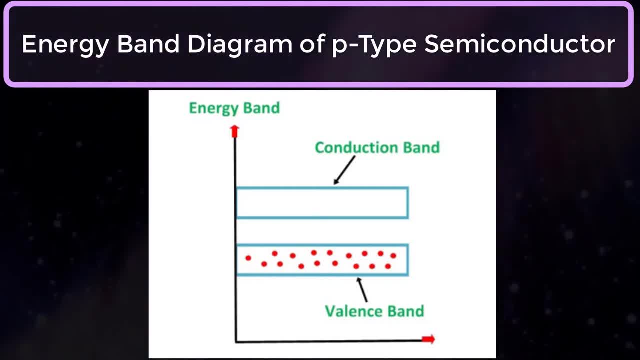 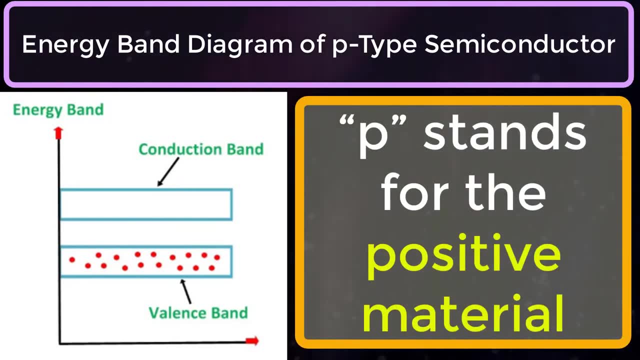 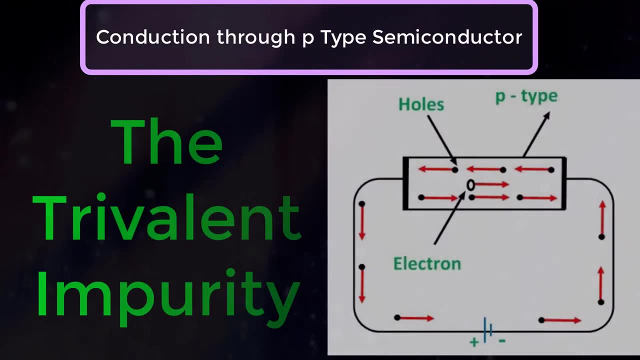 in the conduction band. This is because of the predominance of holes over electrons of the material is called as a P-Type Semiconductor. The word P stands for the positive material Conduction through P-Type Semiconductor. In a P-Type Semiconductor, large number of 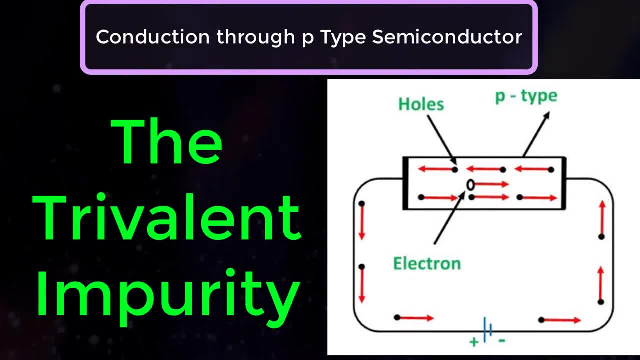 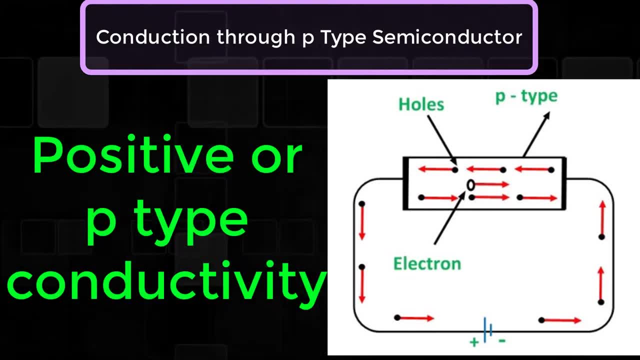 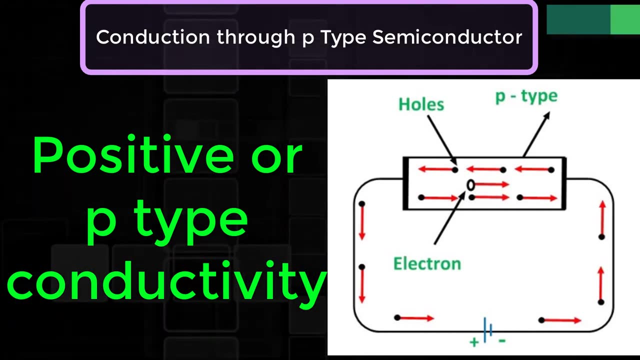 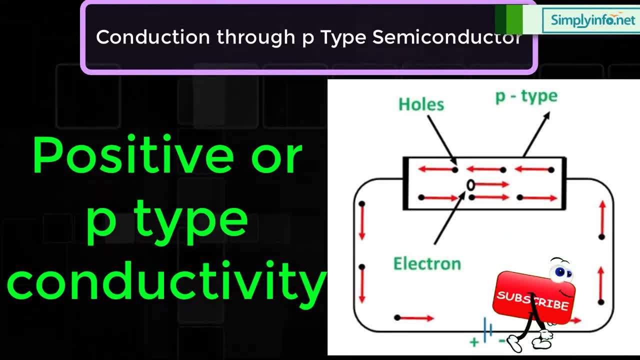 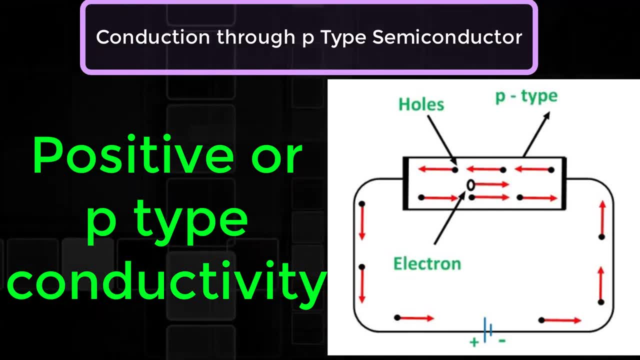 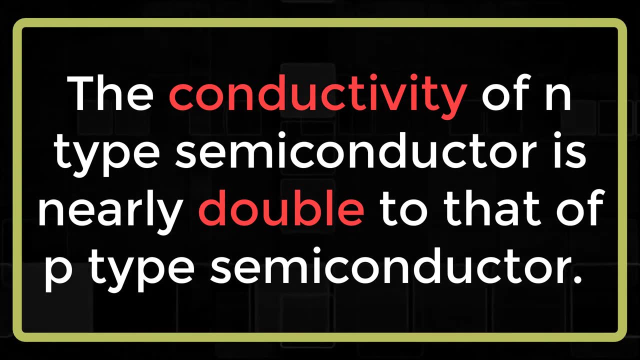 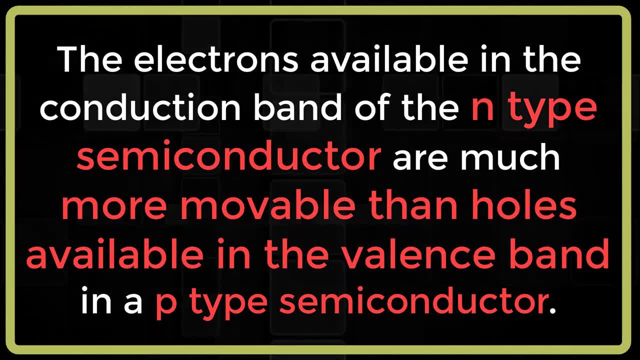 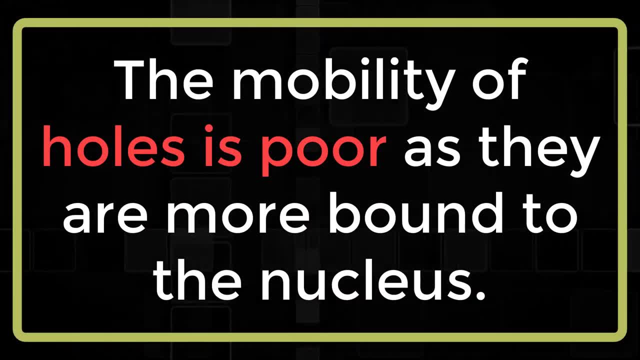 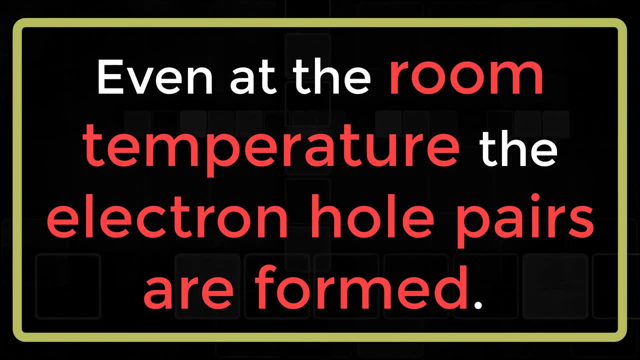 available in the conduction band of the n-type semiconductor are much more mobile than the holes available in the valence band in a p-type semiconductor. the mobility of holes is poor as they are more bound to the nucleus, even at the room temperature. the electron holes spares are available. these free.